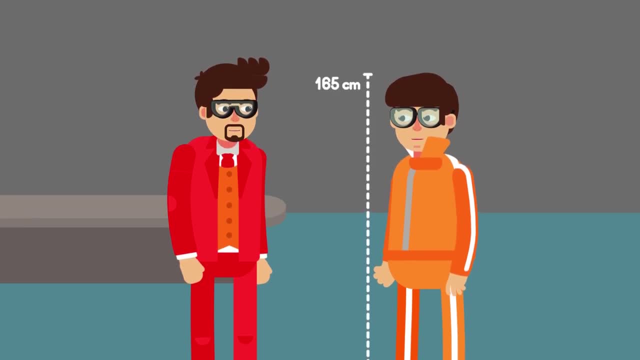 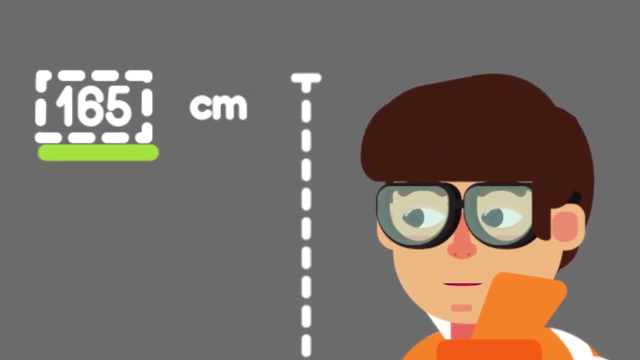 If we say that the height of a student is 165 cm, then it is representing both the properties of a physical quantity. ie 165 is the numerical magnitude, while cm is the unit in which the height is measured. Remember, if we only state height as 165, then it is not a physical quantity, since it does not tell us about the unit in which it is measured. 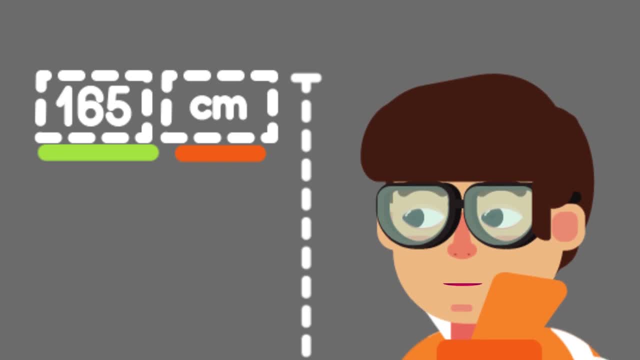 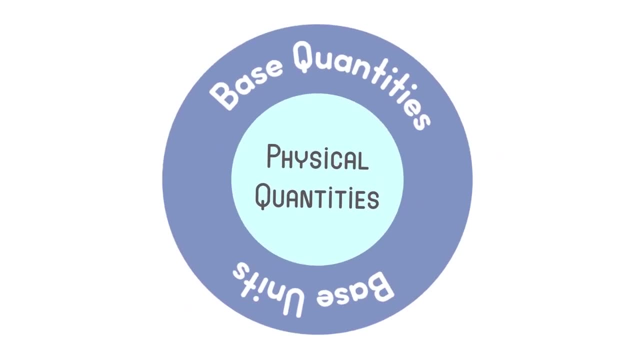 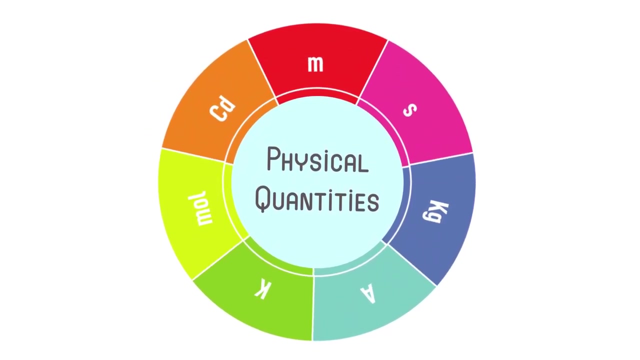 So it is a must for physical quantity to have both magnitude and height. Physical quantities are divided into two categories. Base quantities form the base or foundation of other physical quantities. In other words, the quantities are the basis with which derived quantities are expressed. 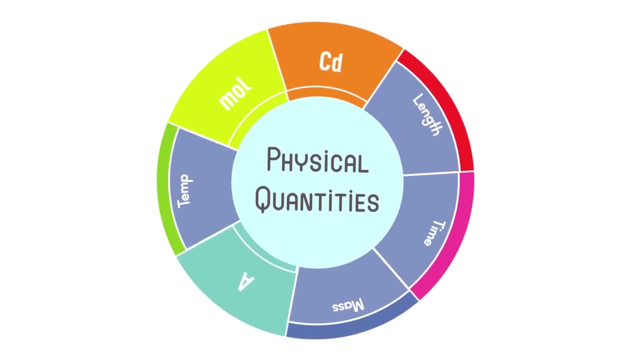 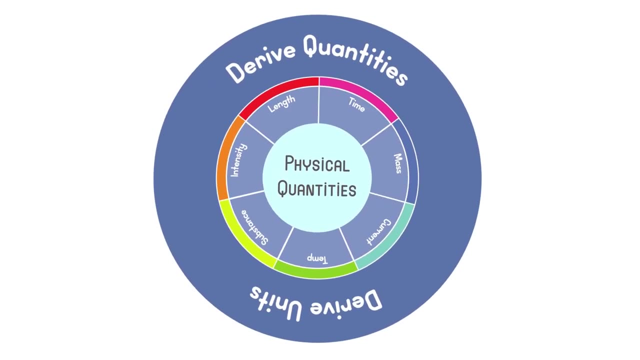 These quantities are length, mass, time, temperature, intensity of light, electric current and the amount of a substance: Derived quantities. Derived quantities, therefore, are the basis with which derived quantities are expressed. The basis quantities are those which are expressed in terms of base quantities. 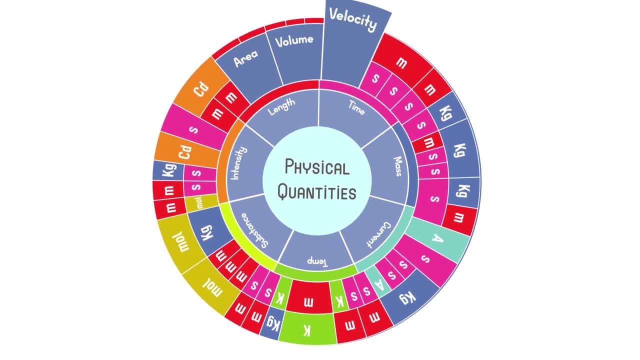 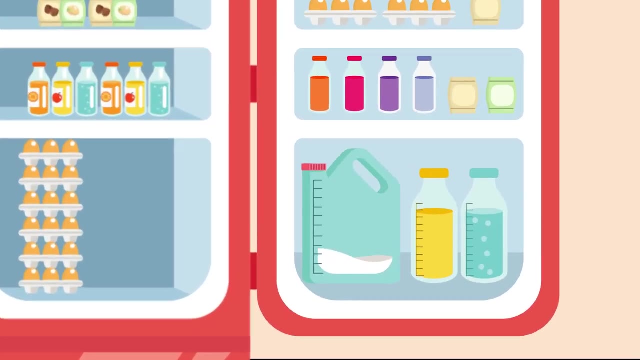 These quantities include area, volume, velocity, acceleration force, pressure, momentum, electric charge, electric induction, etc. Before talking about the units which are associated with base and derived quantities, we need to know about the universally adopted system of units for physical quantities. 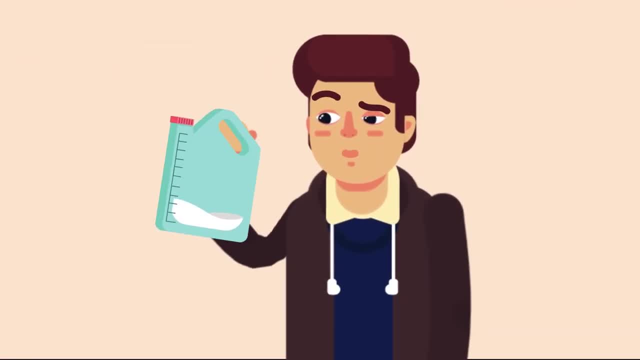 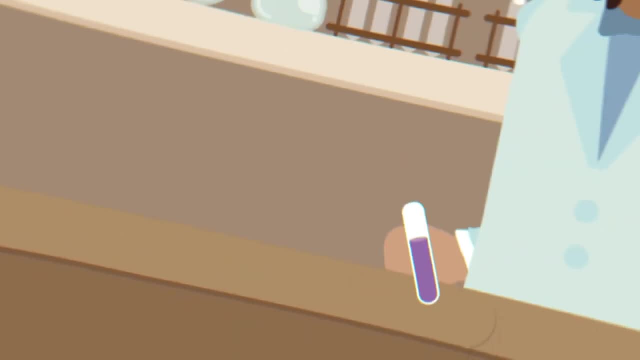 This is to be noted that measuring does not always involve counting. Like if we need milk, we need to understand what quantity of milk is required. Similarly, to describe the physical quantities, a standard is required with which the quantities could be compared and expressed. 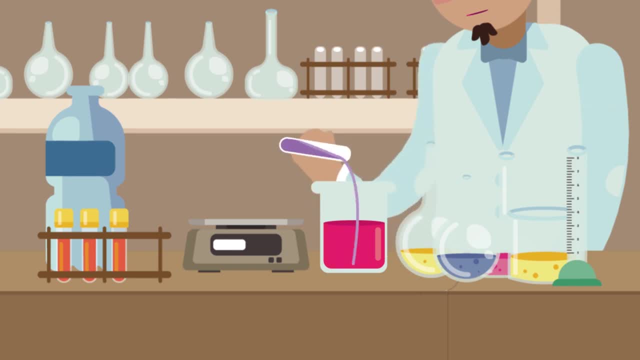 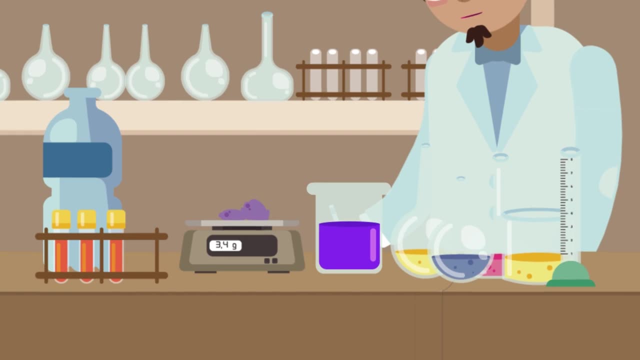 This standard in physics is known as a unit. By that time, it was crucial so that the knowledge and findings, with the advancement of fields, could be shared universally by adopting some known standards. In this context, during the 11th General Conference on Weights and Measures, 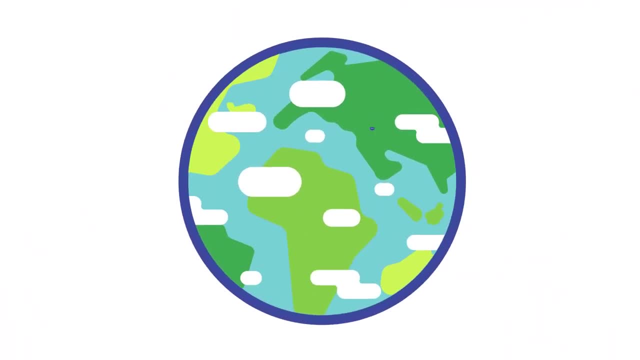 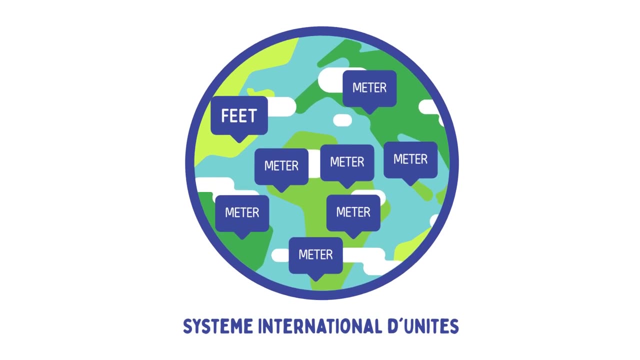 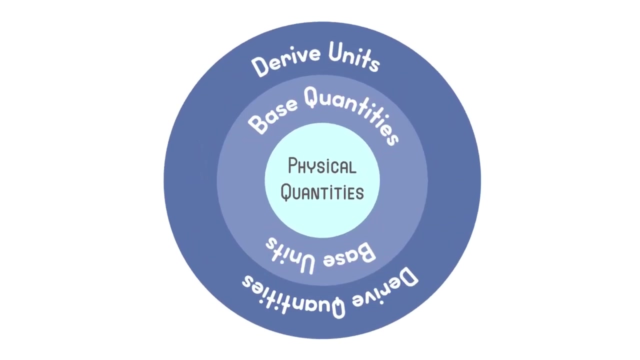 held in Paris in 1960, a universal international system of units was accepted. This system is commonly referred to as SI System International. Now, coming back to the base and derived quantities. we have understood about these quantities. Now we will have a look at the units in which these are measured. 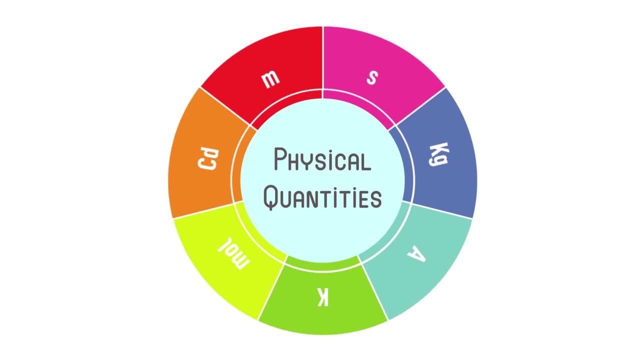 Base units. The units used to measure base quantities are called base units. We now know that base quantities are 7 units, 7 in number. But in what units these quantities are measured? Well, length quantity is measured in meter. Time is measured in second. 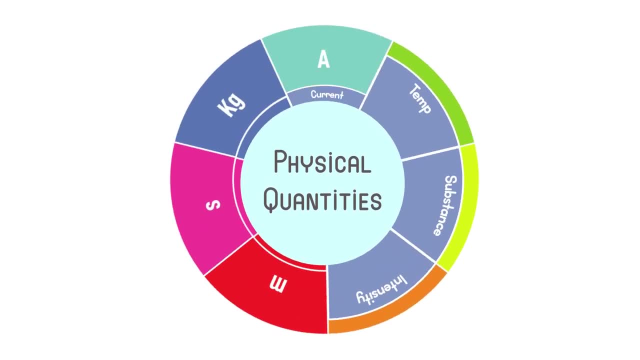 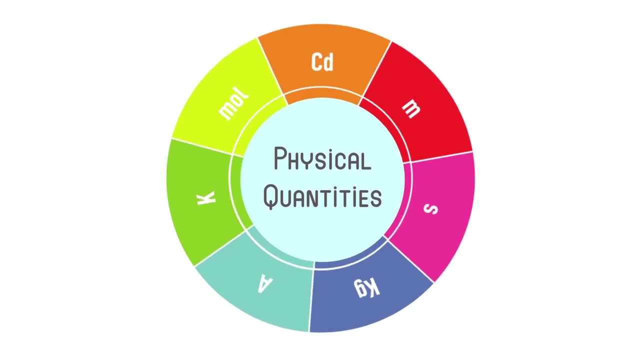 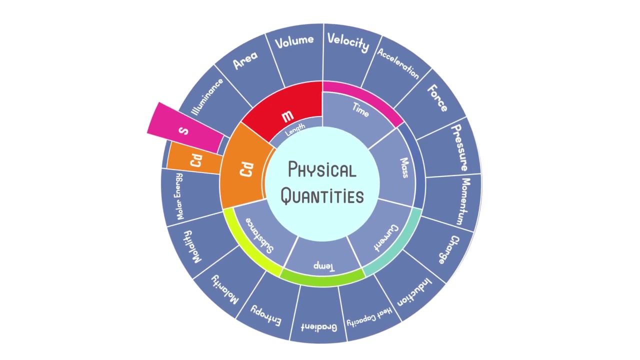 Mass in kilogram, Electric current in ampere, Temperature in kelvin, Amount of substance in mole And intensity of light in candela. Derived units. The units used to measure derived quantities are called derived units. They are defined in terms of base units. 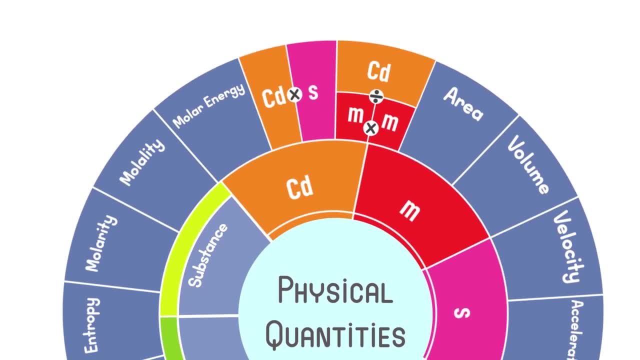 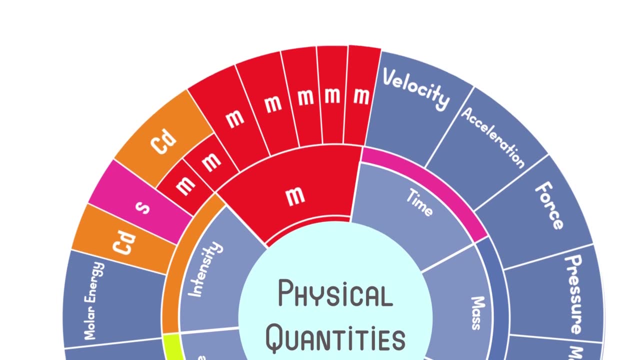 We get them by multiplying all the units Or dividing one or more base units with each other. For example, the unit for area is square meter And for volume is cubic meter, which are based on the unit of length. Some derived units and their symbols are as follows. 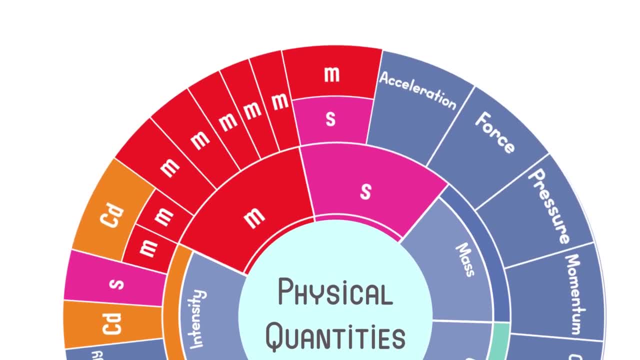 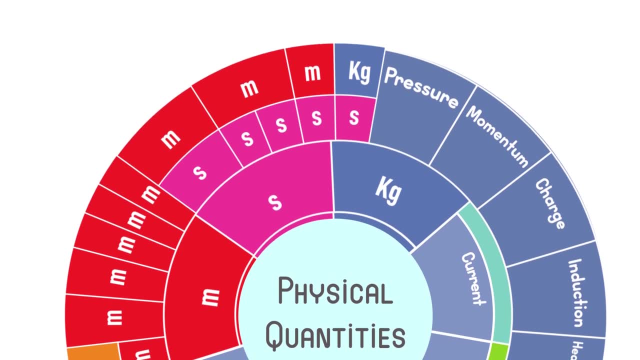 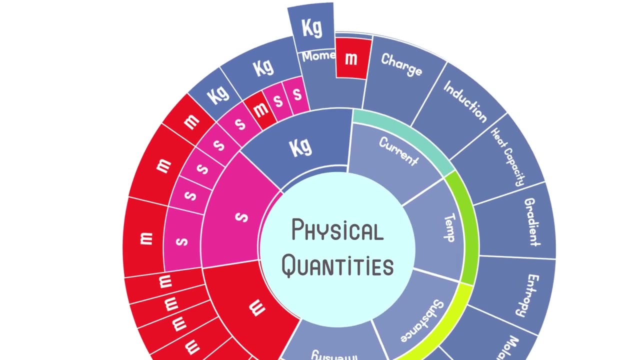 Velocity, which is measured in meter per second. Acceleration measured in meter per second. squared. Force in meter kilogram per second squared, Or termed as Newton Pressure in Pascal Or kilogram per meter second squared. Momentum in meter kilogram per second. 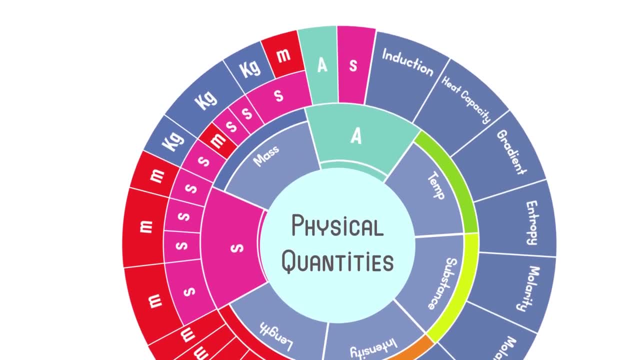 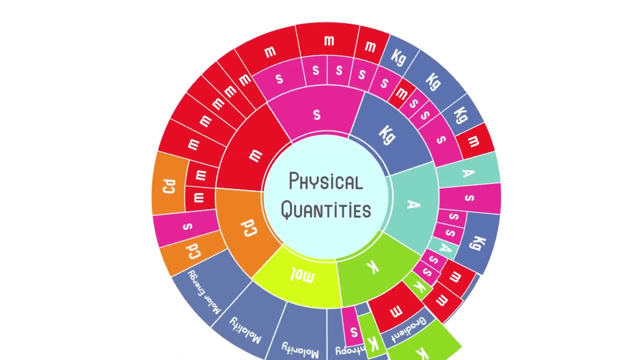 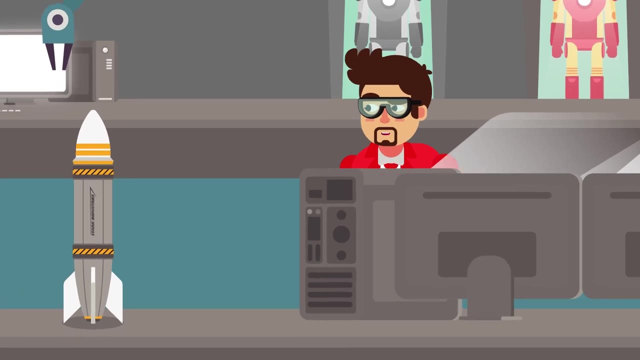 Charge in coulomb or ampere second, And magnetic flux density in Tesla Or kilogram per second squared ampere. Let's take a deeper look into these. How can we measure quantities like lengths with proper accuracy? There are several ways. 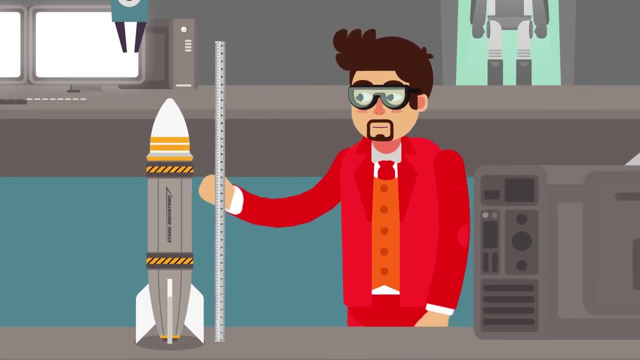 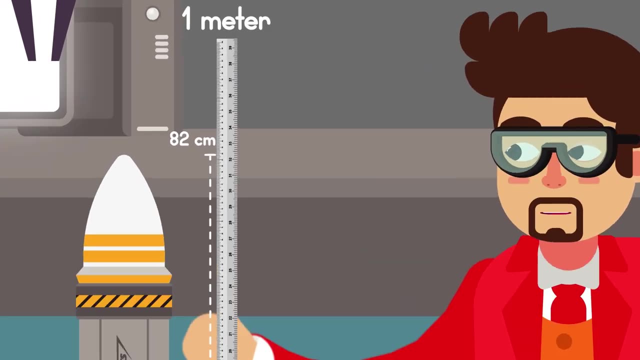 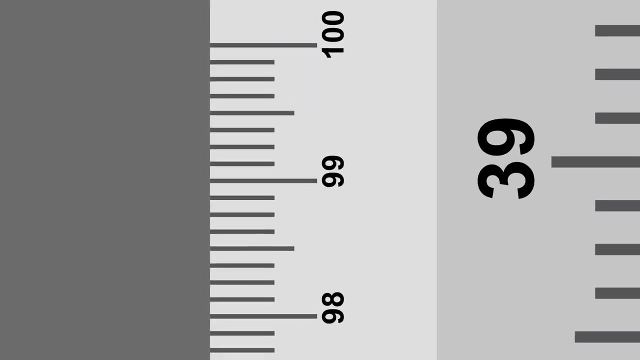 Meter rule. It is used to measure the length or distance between any two points. As the name indicates, it is one meter in length, which, by convention, divided into 100 centimeters. Each centimeter consists of ten small divisions, known as millimeter. 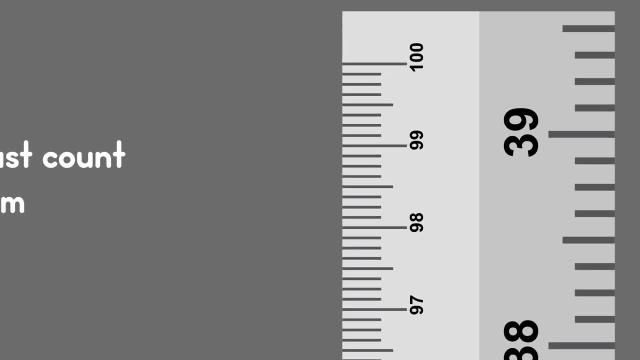 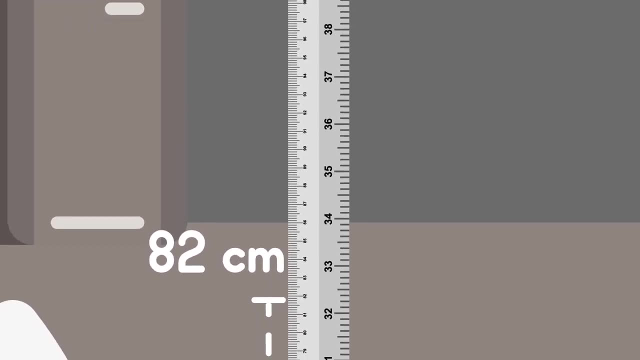 Thus, the smallest reading that a meter rule can give is one millimeter, Also known as its least count. To have accurate measurements using a meter rule, we must keep our eyes directly above the rule. We must keep our eyes directly above the reading points. 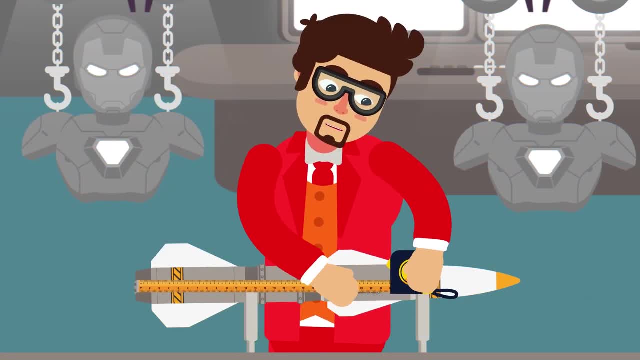 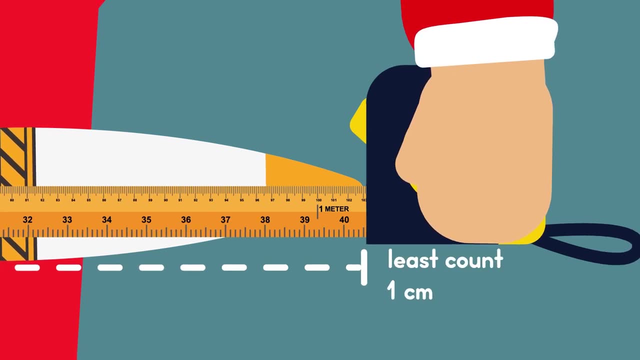 Measuring tape. It is used by carpenters and builders to measure a greater length, usually in meter, centimeter and inches. This means one centimeter is the least count of measuring tape, The same as in meter rule To measure accurately using a measuring tape.